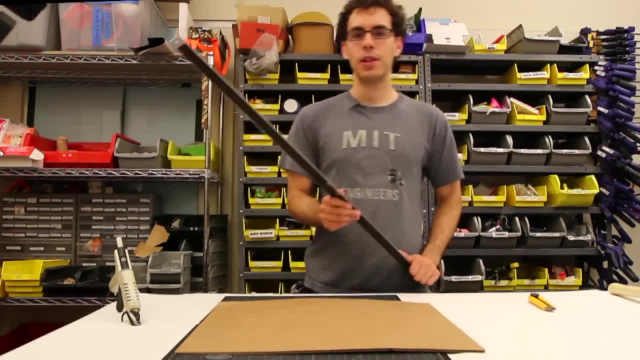 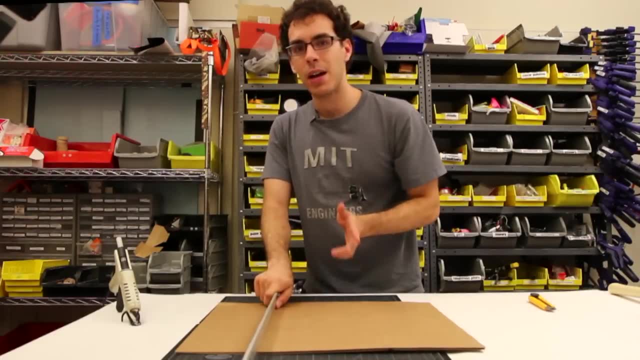 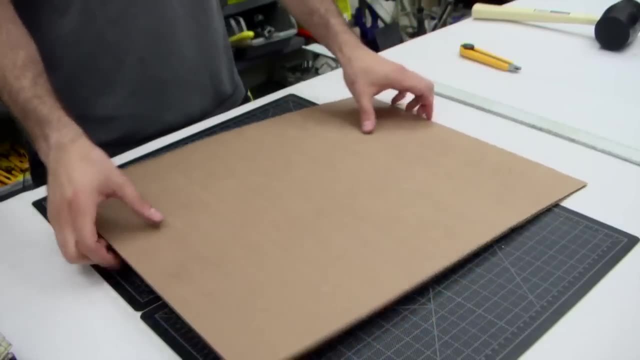 thing that we're going to do is bend the cardboard, and for that we're going to use a straight edge. You use the straight edge to make a dent in the cardboard, but if it's too hard to make a dent, it helps to have a rubber mallet handy. So with just a whack you've. 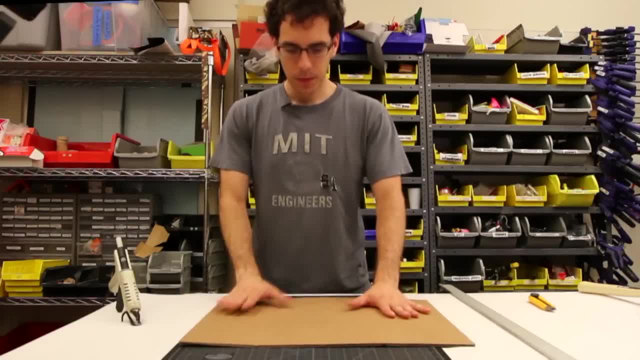 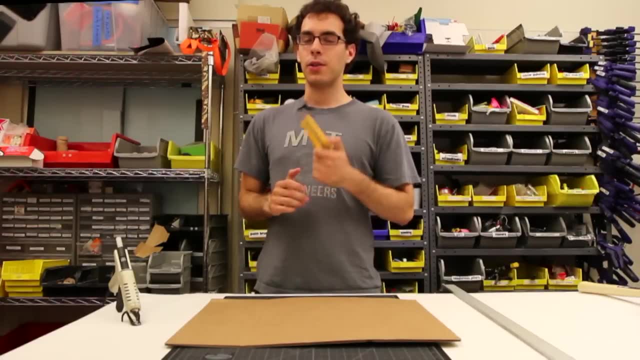 got a nice clean bend. Now the next thing that we're going to go over is cutting cardboard with a utility knife. Now you have to be careful. These knives are incredibly sharp and that makes them one of the most dangerous tools in the shop If you're not comfortable using. 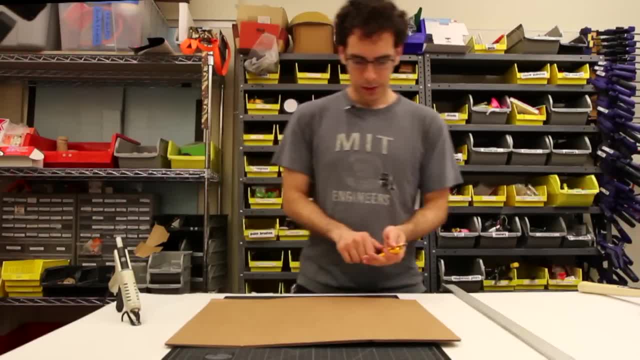 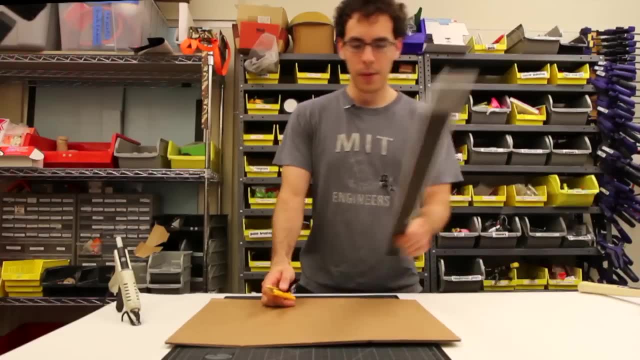 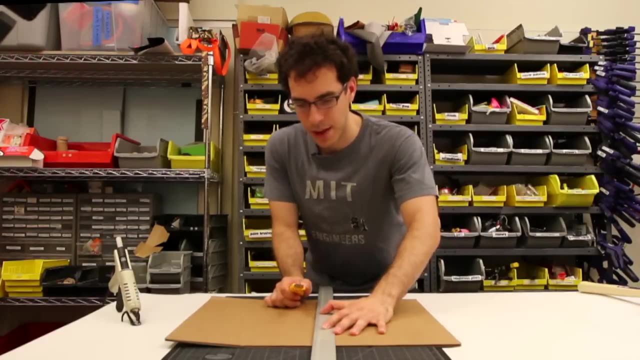 one, then ask someone to give you a hand. One tip is to keep the blade retracted until you're going to use it. That way, nobody accidentally picks it up with the blade and you don't want to get hurt. Now, one safe way to make a cut is to pretend that your fingers have. 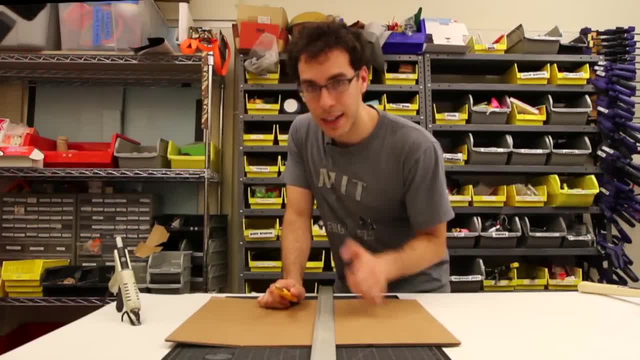 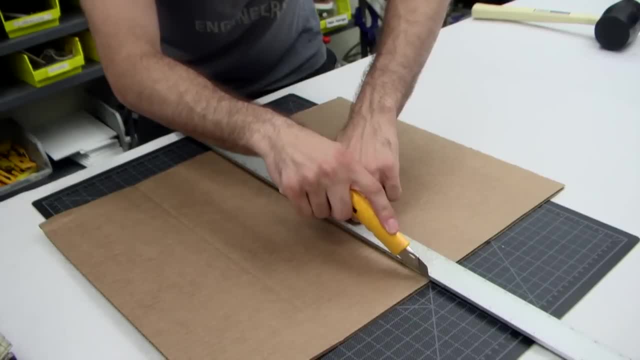 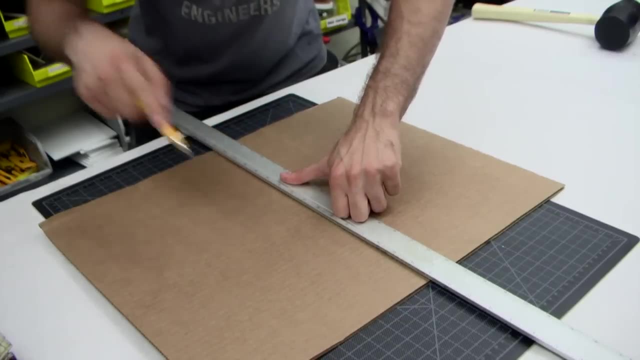 already been cut off. That way they're not going to stick out and get in the way of the cut. Then you just take your blade, you place it up against the straight edge and with a low cutting angle like this, not like this- you make a few gentle passes. Now you want. 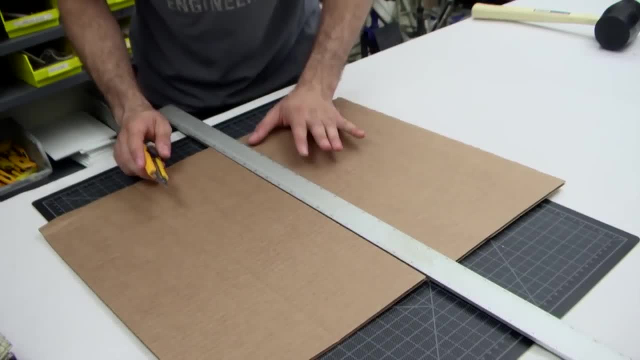 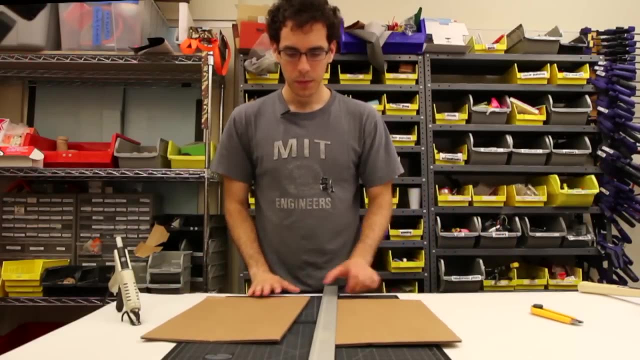 to use gentle passes, so that way, if you slip, you're going to get hurt. You want to make sure that you don't do any major damage? Go ahead and put the blade away and we've got a nice clean cut. The last thing that we're going to do is we're going to join pieces. 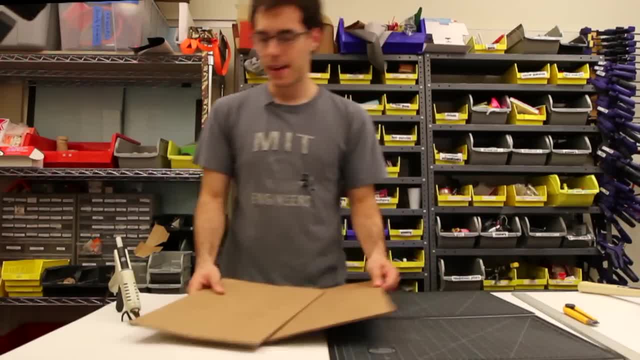 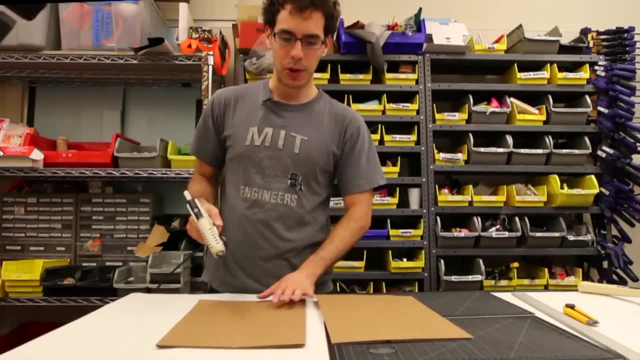 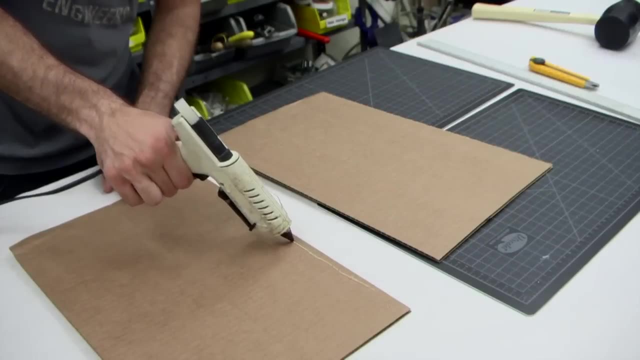 of cardboard together, and one tool that's great for doing that is a hot glue gun. Hot glue dries pretty quickly and that makes it pretty nice for putting prototypes together. It's also great for joining cardboard. It's really going to stick it together well, So 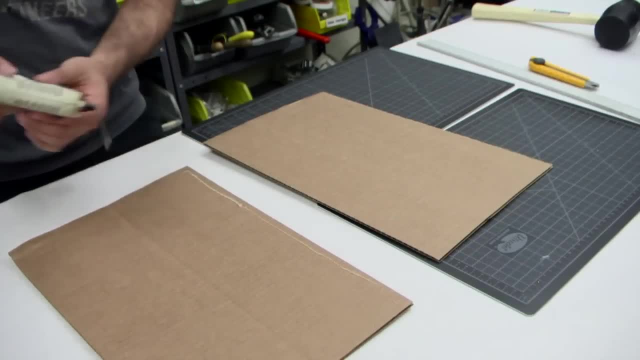 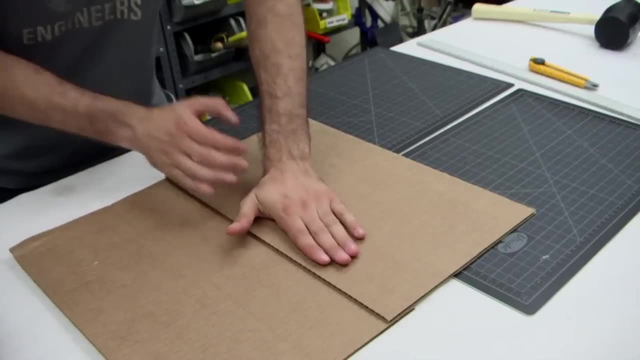 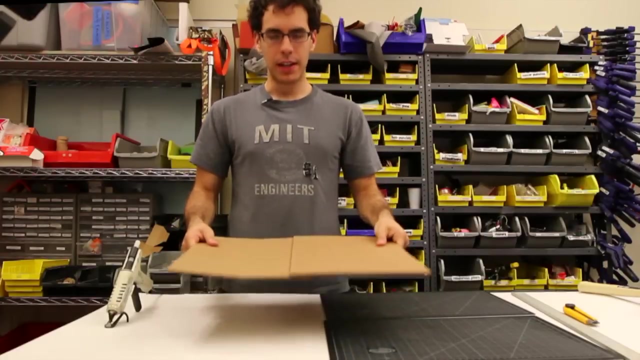 you want to get one solid bead down, press the sheets of cardboard together and wait for about 10 to 15 seconds, and then you've got a nice strong joint. So now let's take these techniques and put them together to make a prototype. 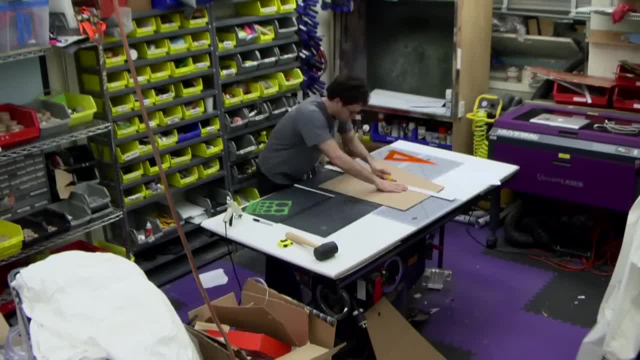 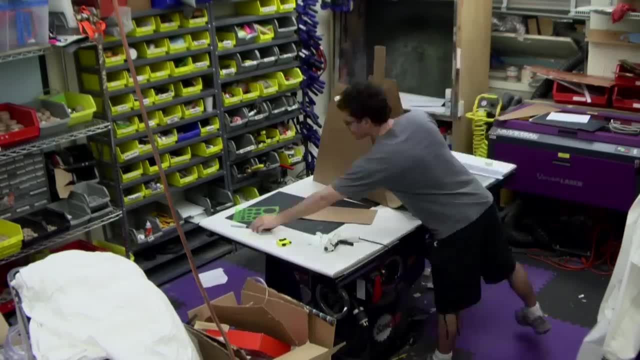 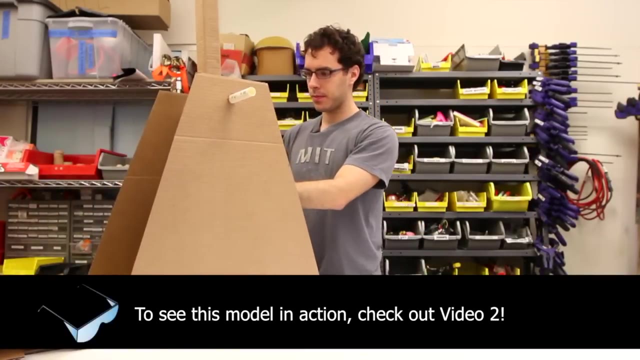 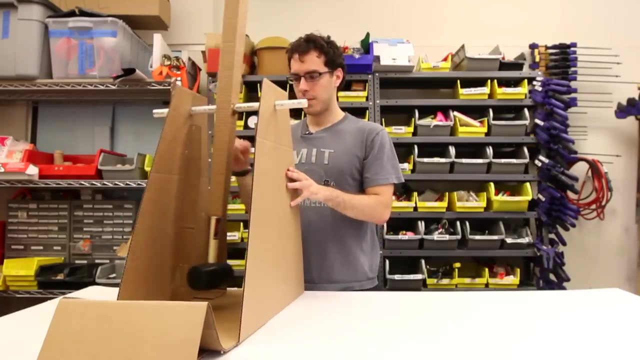 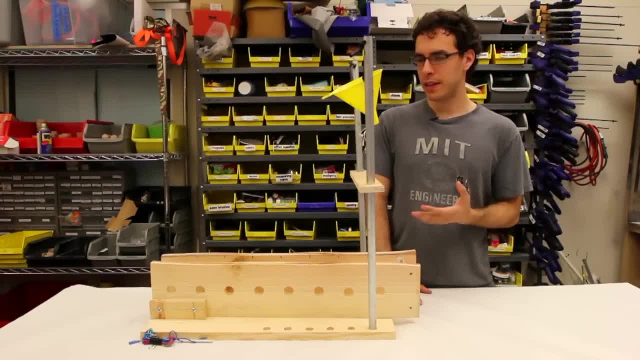 On the other side of the jos. kurz, I'm going to look for a space for Seeing. óthis will be our new hepatritt option on our amazing Maserati 365: Food. the new Tears- луч jibee- the new Tears. close-up on our Japanese F-250ucking race car. 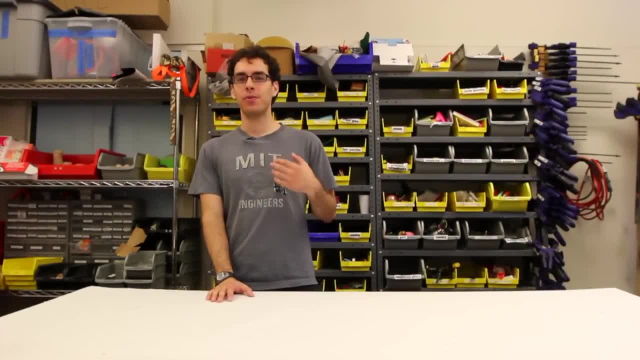 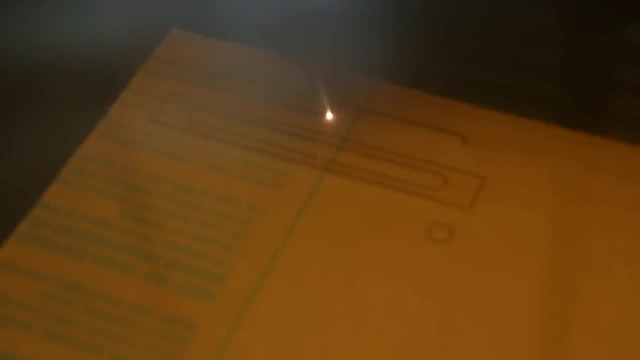 And I'm going to cut it out and I'll put it from there. OK, And I'm going to cut it out. that help you make prototypes really quickly. We have a laser cutter which uses a powerful beam of light to cut sheets of materials like wood and plastic.